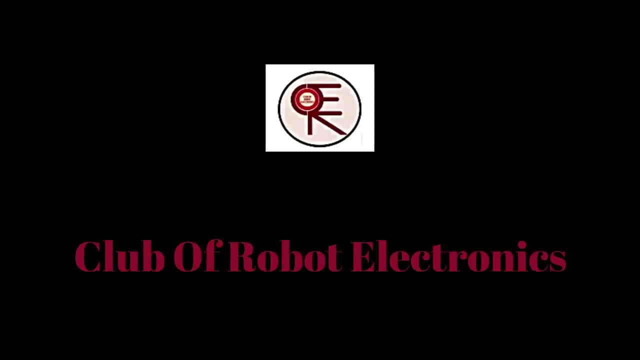 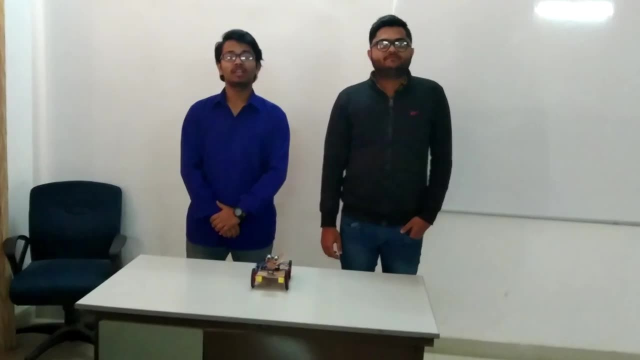 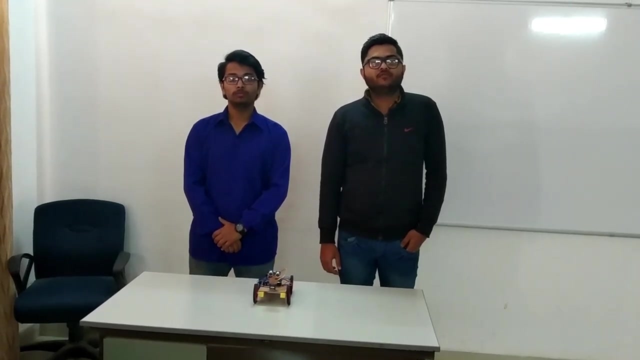 Hello everyone. my name is Pranshu Bajpayee. My name is Ayush Gautam. We are from Club of Robot Electronics in College of Technology and Engineering, Udaipur, Rajasthan. We are here to present you this project, which is based on Arduino Uno. This is the obstacle: avoiding robot. 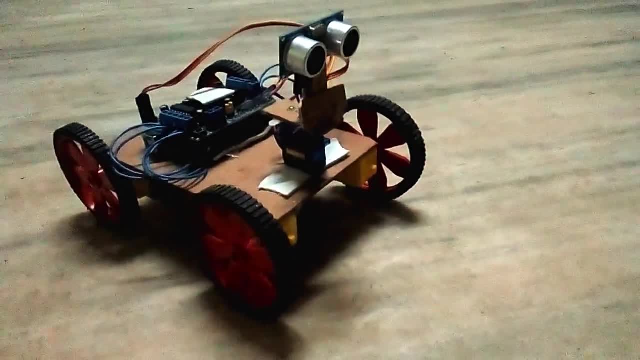 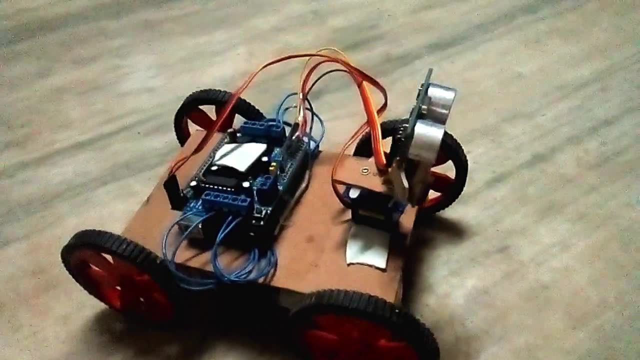 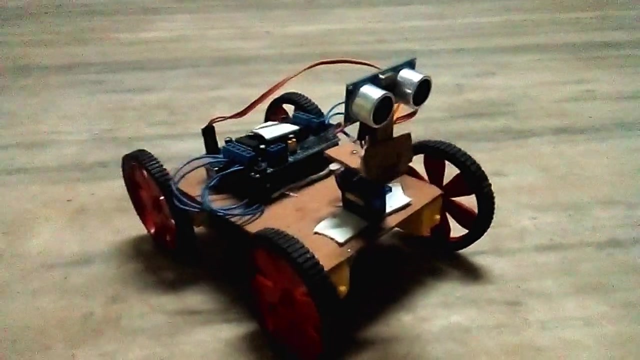 Obstacle avoiding robot is an intelligent device which can automatically sense the obstacle in front of it and avoid them by turning itself in another direction. This design allows the robot to navigate in unknown environment by avoiding the collisions, which is a primary requirement for any autonomous mobile robot. 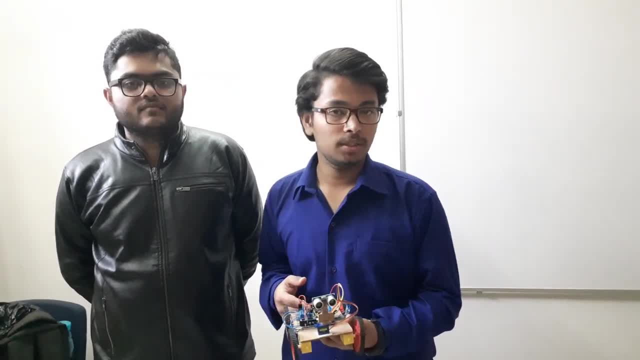 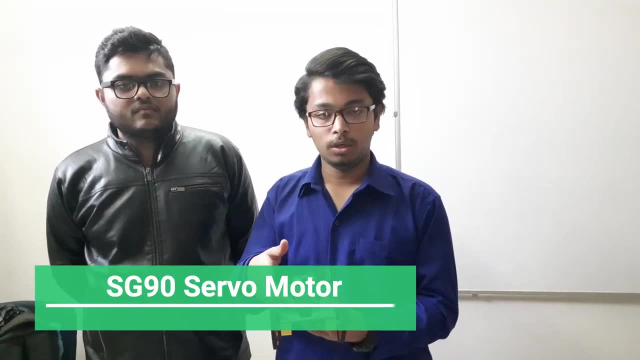 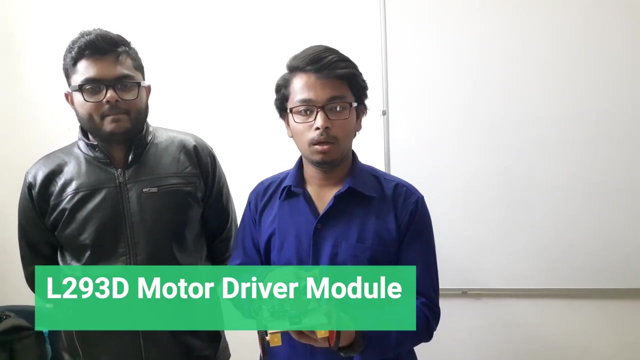 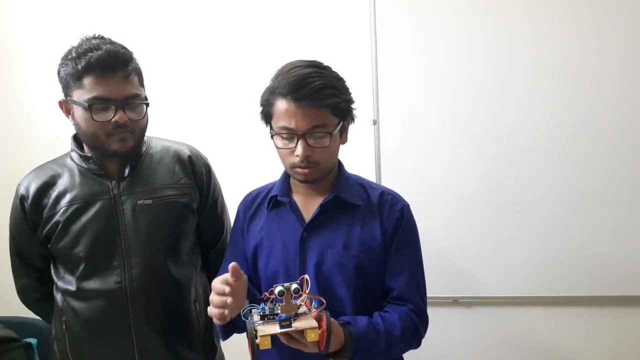 Components required for this obstacle avoiding robot can be found very easily. The first component we require is the HCSR04 ultrasonic sensor, Then we need the SG90.. We need 4 wheels, 4 gate motors, then we also need an Arduino Uno board, then we need L293D motor driver module. we also require 2 9V batteries, battery holder, jumper wires and that's all. 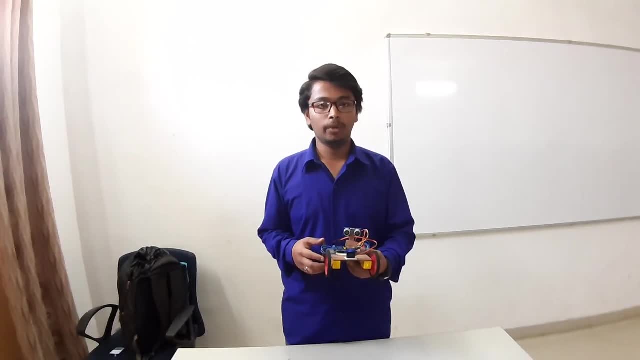 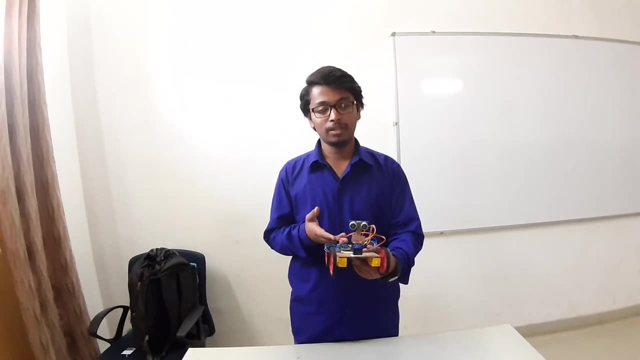 Now we have to understand what are the components used in this obstacle avoiding robot. The first component used is the Arduino Uno board. It is the main component used in this project, as it is also known as the heart of this project. This is the Arduino Uno board. 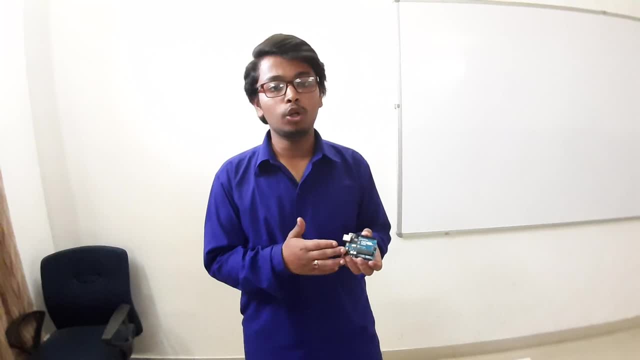 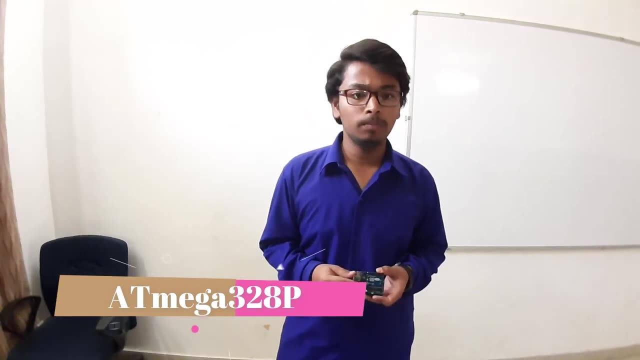 Well, all the coding is done in this and you can see that it controls all the activities of this obstacle avoiding robot. So basically, Arduino Uno is an ATmega328p macro controller based prototype robot. It is an open-source electronic strategy platform that can be used with various sensors and actuators. 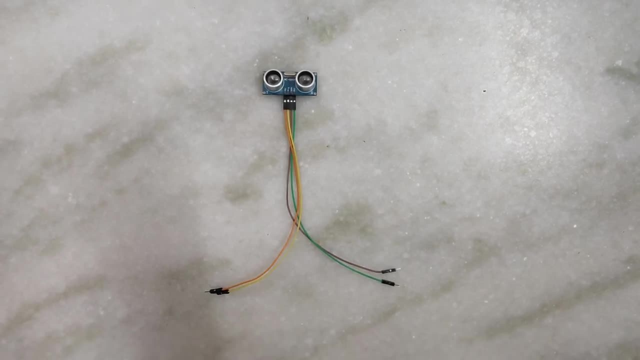 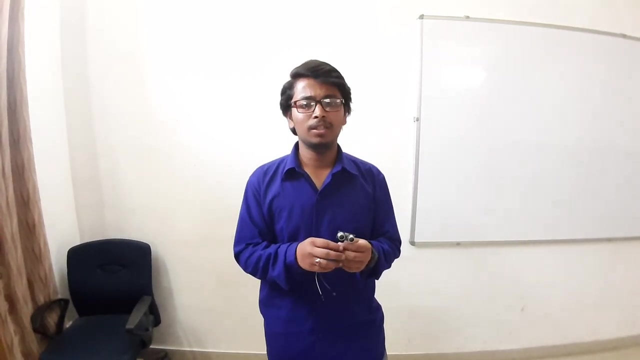 The next component is the HCSR04 ultrasonic sensor. Well, to understand it easily, you can really say the distance between the obstacle and the robot And some of the coding is done accordingly. so this robot has to stop about 2 cm from the obstacle. 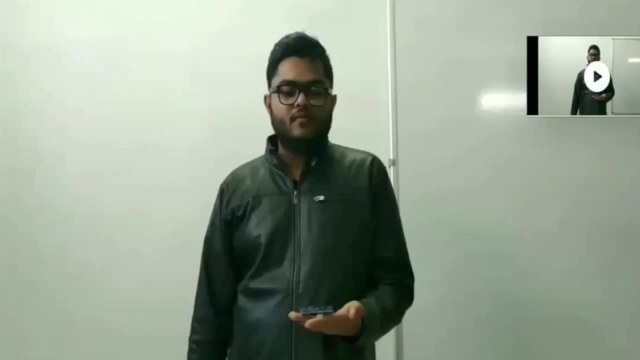 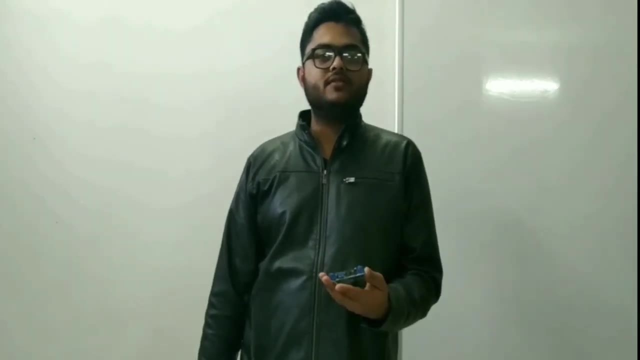 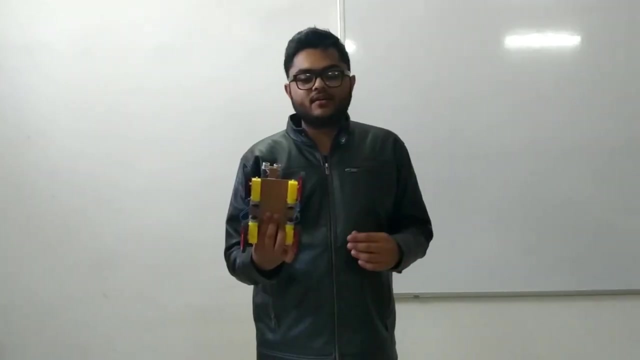 5 centimeter or 10 centimeters according to the needs. the next component which we are using in our obstacle avoiding robot is L293D motor. L293D motor consists of two H-bridge. H-bridge is the simplest circuit for controlling low circuit rated motors. the next component of our obstacle avoiding robot.